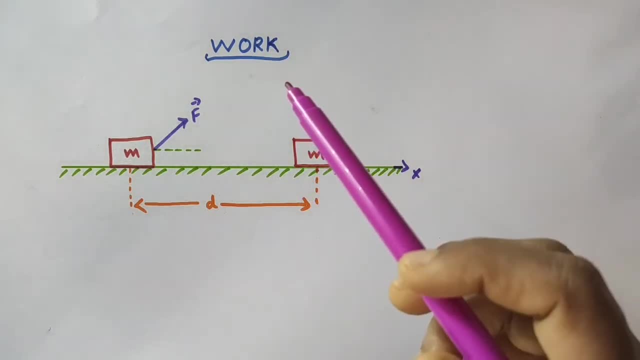 that In this video we are actually talking about the work done by a constant force, That is, the force is constant throughout the motion of that object we are considering. Okay, so here you just consider an object of mass m. It is kept on a surface. Okay, now consider a constant force. 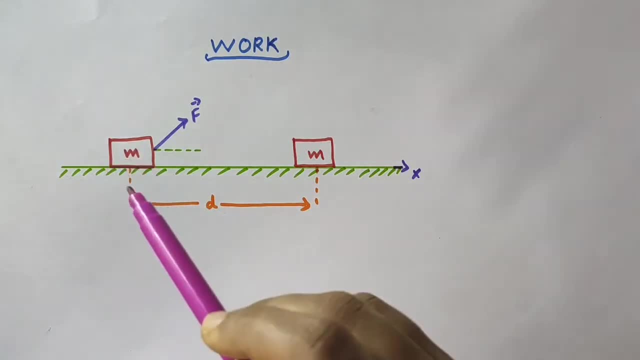 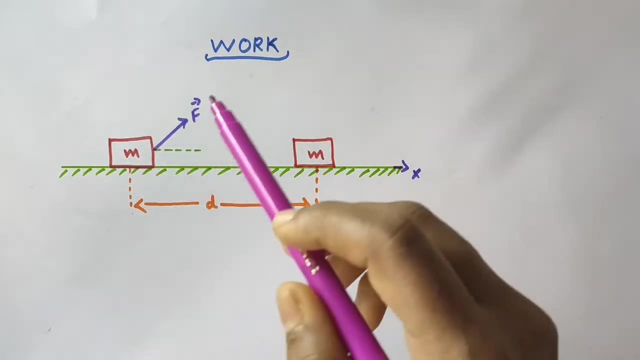 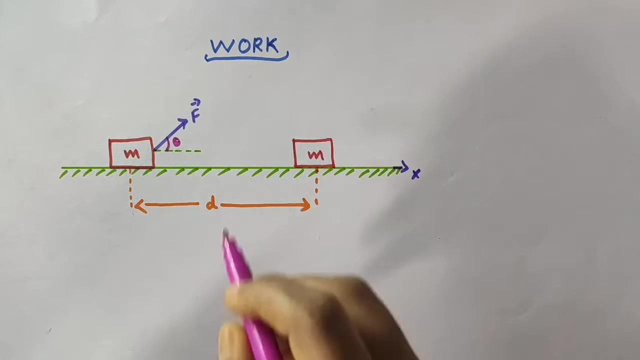 vector F acting on this object of mass m. Okay, that is a constant force. vector F is acting on this object of mass m and you can see that this force is acting in a particular direction, which makes some angle theta with the horizontal direction. Okay, this dotter line is actually. 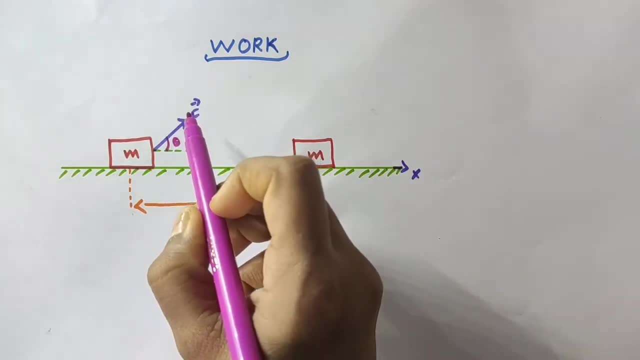 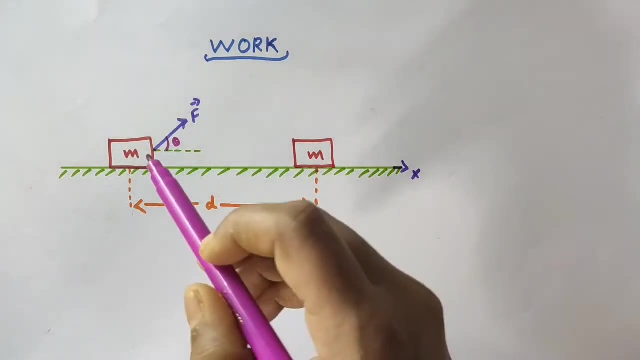 parallel to the surface. now. So we can say that this force is acting on a particular direction which makes some angle theta with the horizontal force, is actually making some angle theta with the surface where the object is kept. Okay, now, because of the force acts on this object, let the object undergoes a displacement. 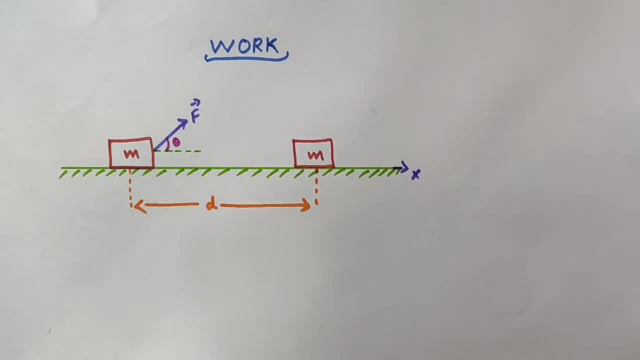 d. Okay, this can be taken as vector d. So let the object undergoes a displacement. vector d: along the positive x direction. So this is along the positive x direction. Okay, the object was here at first, but under the influence of the force it undergoes a. 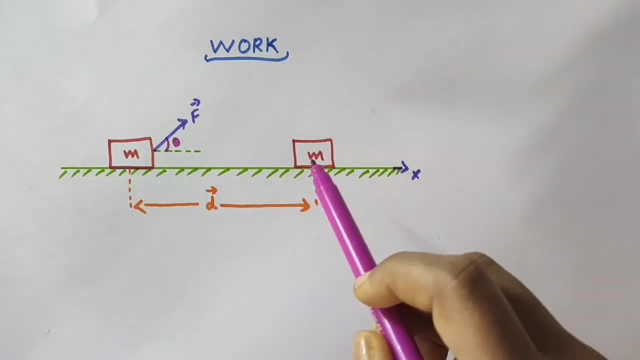 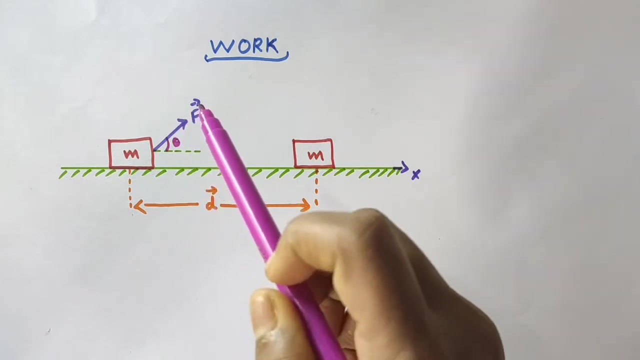 displacement vector d and reaches here after sometime. Okay, here you see the direction of the displacement vector d. it is along the positive x direction. Okay, but the direction of force is like this. That is this force vector f that makes an angle theta with the positive x. 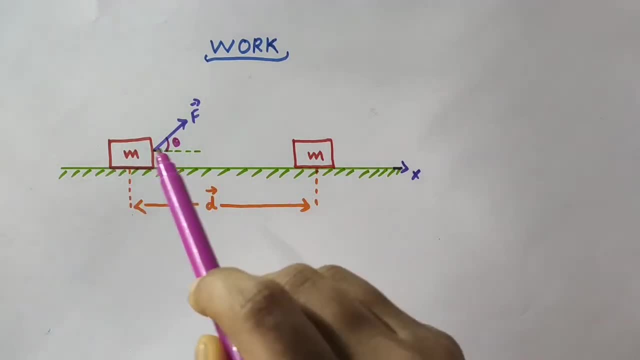 direction. This dotted line is like this. So this is along the positive x direction. This dotted line is actually parallel to the surface. This dotted line is actually parallel to the positive x direction. So we can say that theta is the angle between the force direction. 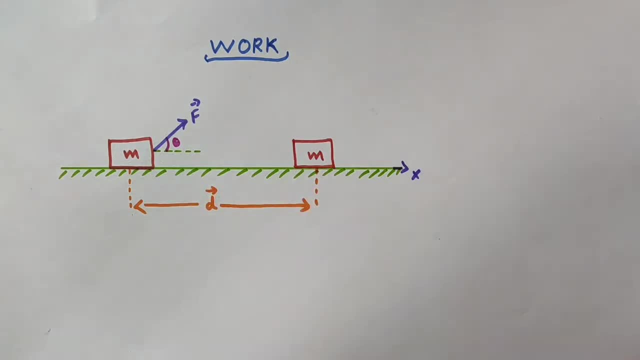 and the positive x direction. Now you see, we have studied about resolution of vectors in our previous videos. no, So while we have talked about that resolution of vectors, actually we can resolve this vector f into two component vectors. no, That is, we can resolve this force. 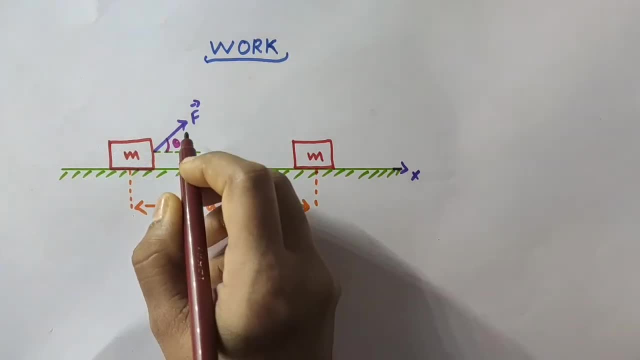 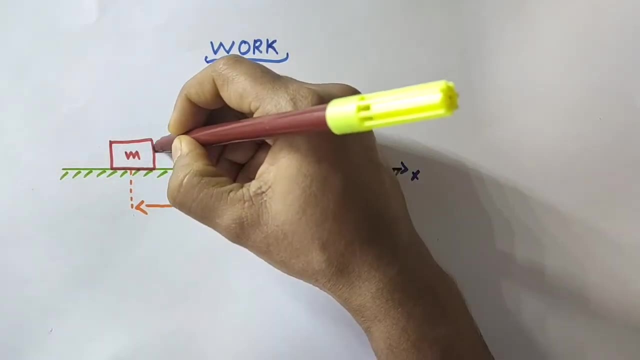 vector into its two components, So we can resolve this force vector into its two components, two component vectors. so i'm just, i mean we can resolve this force vector into one horizontal component and we can resolve this vector into f, into one. i mean it will have one vertical component. 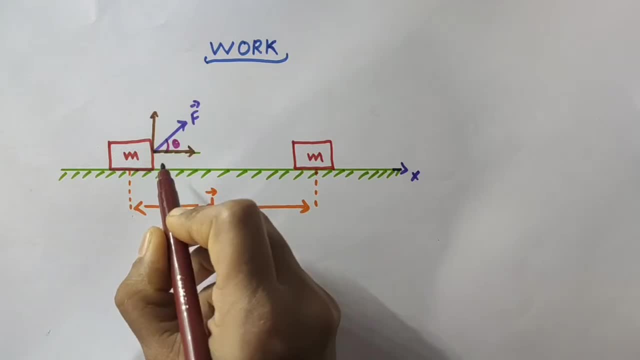 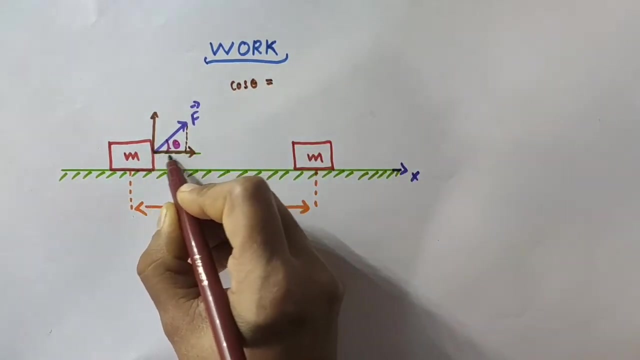 and it will have one horizontal component. so what about the horizontal component of this force? that is, we just want to form a triangle here. this is theta, so a horizontal component means this component. so i'm just calculating cos theta. cos theta is equal to adjacent side, adjacent side. 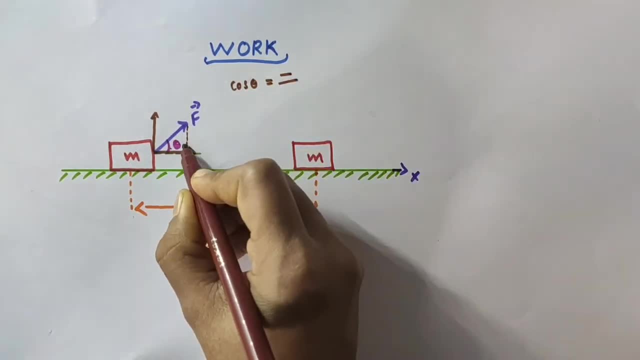 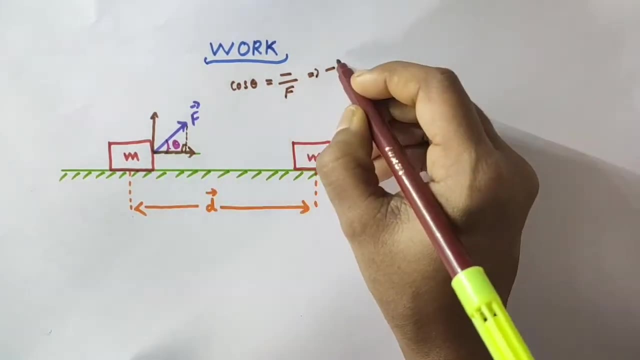 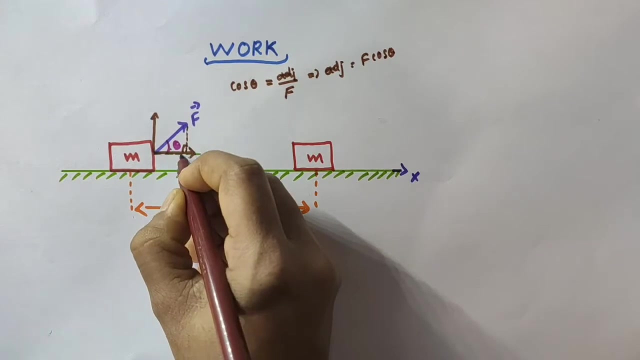 means this side, okay, that side, divided by hypertenuse, this is 90, so hypertenuse that has a magnitude f so f. so that side, that is this adjacent side. okay, i'm writing it as adjacent side. so adjacent side is equal to what? f cos theta? all right, so this f cos theta is actually. 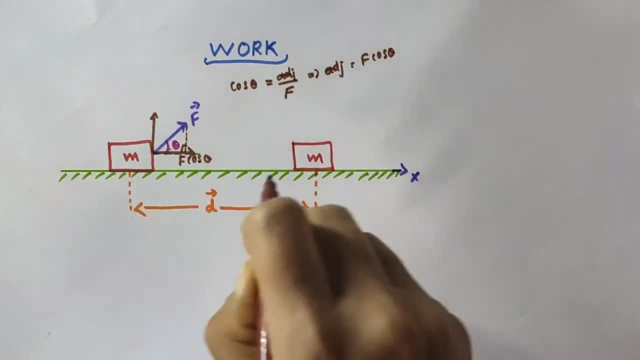 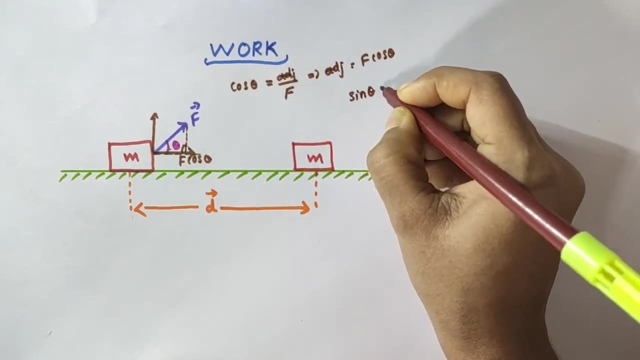 the component of the force in the direction of displacement or in the positive you x direction. okay, now here, if i'm finding out: sine theta. okay, what about sine theta? sine theta is equal to opposite side. opposite side is this side, okay? opposite side divided by hypertenuse is f. 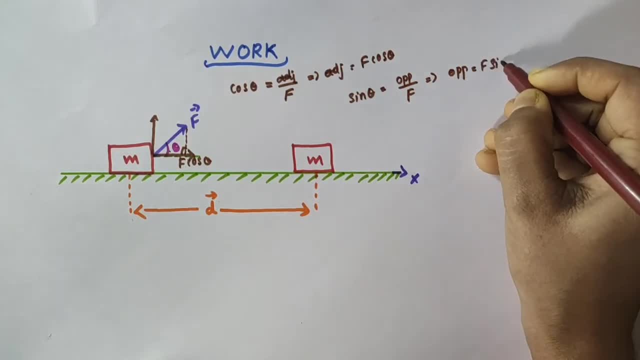 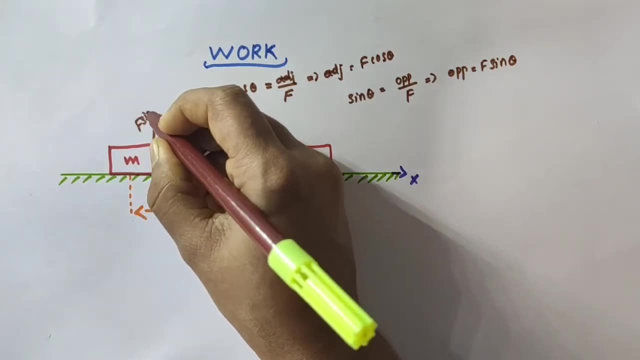 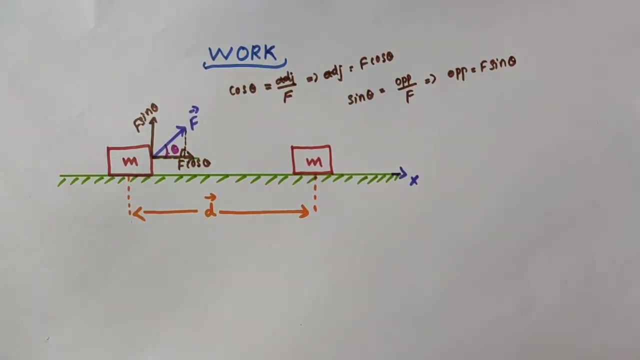 so opposite side is equal to what f sine theta. that is, opposite side means this side. it is actually parallel to this. no, so the vertical component is what f sine theta. okay, now see, you have actually studied about definition of work in your lower classes and you have taken the work done by the force as a product. 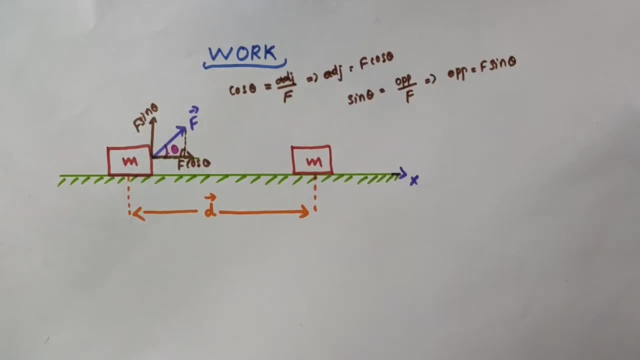 of the force and displacement. but we will take that definition when the force and displacement are along the same direction, when they make an angle theta, i mean an angle theta equal to zero. but here you see, this force is actually acting in a particular direction which makes some angle. 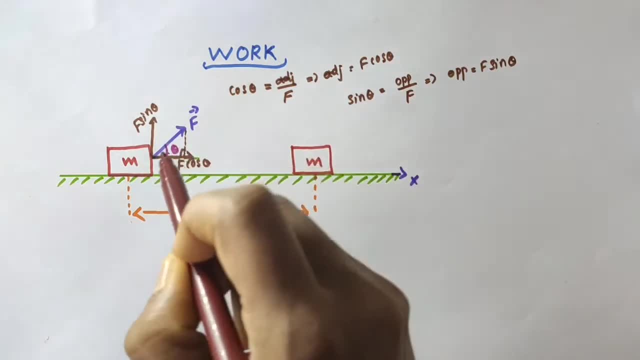 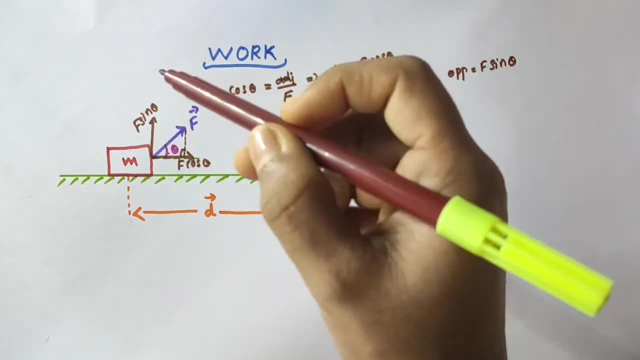 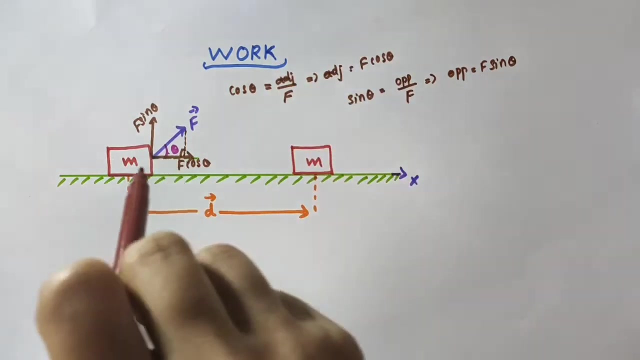 theta with the displacement direction. okay, so this force has two component vectors. one is f cos theta is f sine theta. see this: f sine theta, it is a vertical component. no, since this object doesn't have any vertical motion, which is the force responsible for the motion of this object along. 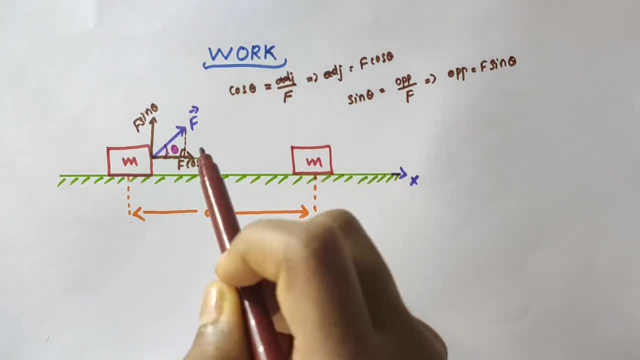 the positive x direction f cos theta. no, because f cos theta is acting along the positive x direction. f cos theta is acting in the displacement direction. so the force responsible, or the component of the force which is responsible, for the motion of this object from here to here, 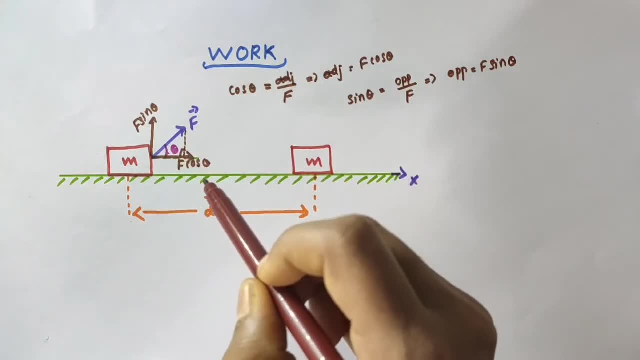 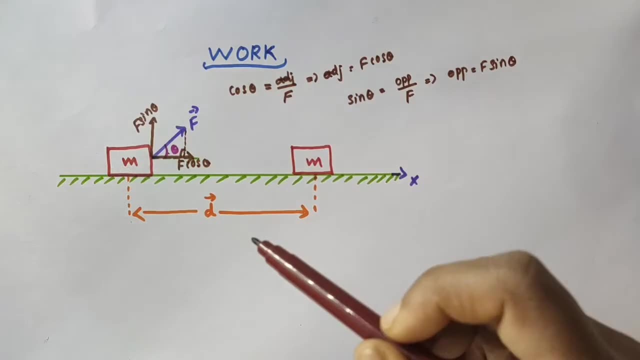 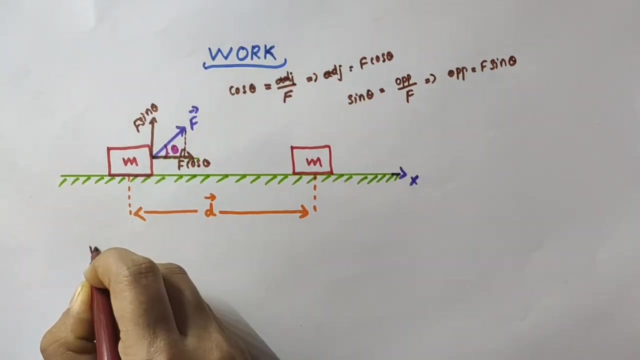 along the positive x direction. is what? f cos theta? okay, we can say that f cos theta is the component of the force in the direction of displacement. okay, now, the work done by the force is defined to be the product of component of this force. so i'm writing: work done. w is equal. 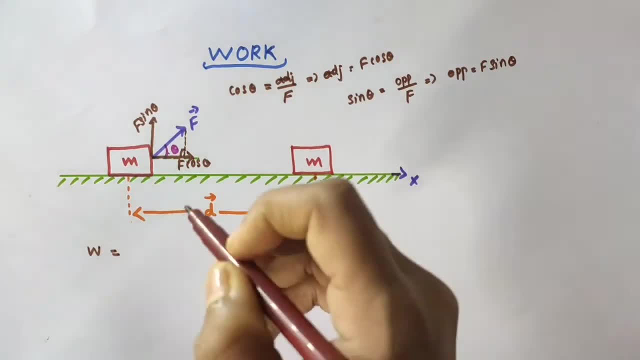 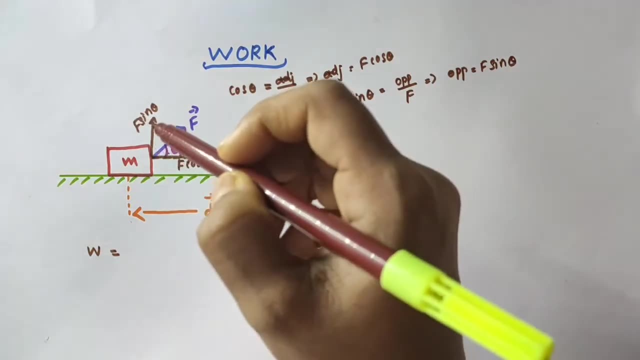 it is defined to be the product of the component of the force in the direction of displacement. the component of the force in the direction of displacement is what? f cos theta, f sine theta is the component of this force, but in the vertical direction. okay, so the component of the force in 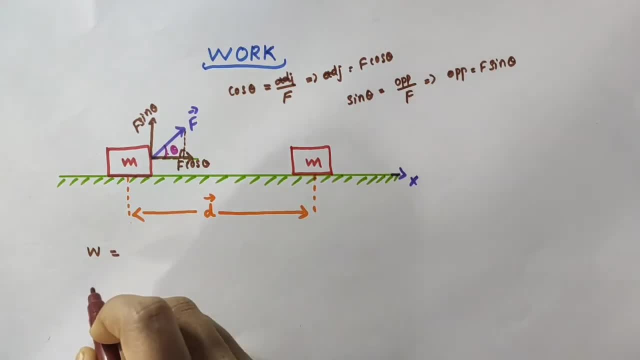 the direction of displacement is what f cos theta. so this work done by the force is defined to be the product of component of the force in the direction of displacement. that is f cos theta and the magnitude of the displacement. what is the magnitude of the displacement? d? okay, this can be. 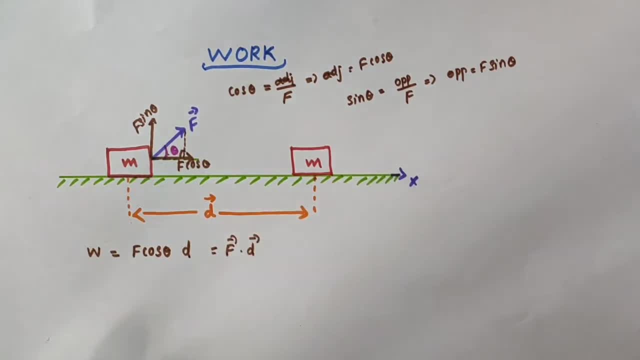 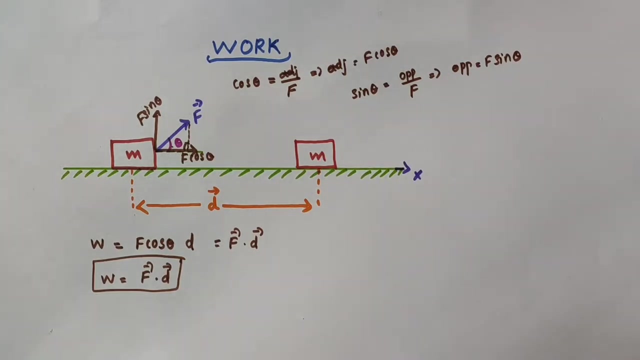 written as vector f, dot vector d. okay, we can write: w is equal to work done is equal to the dot product of the two vectors, the force vector and the displacement vector. no, because when we have discussed about the scalar product or dot product in our previous videos, we define the scalar product between the scalar 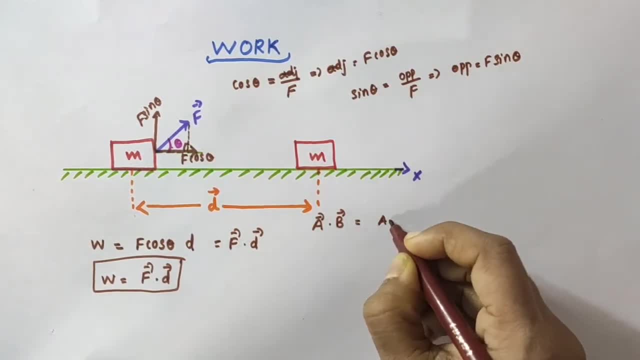 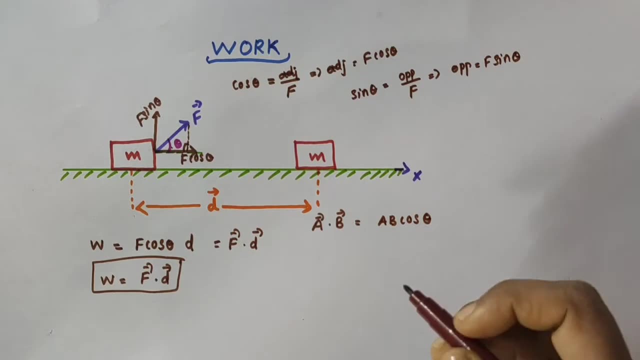 product of two vectors, vector a dot vector b, as a into b, into cos of angle between them. that is, vector a dot b is equal to a b cos theta. okay, i will provide the link in the description box for the description box about that scalar product. you can watch that if you want. okay, so vector a- dot vector. 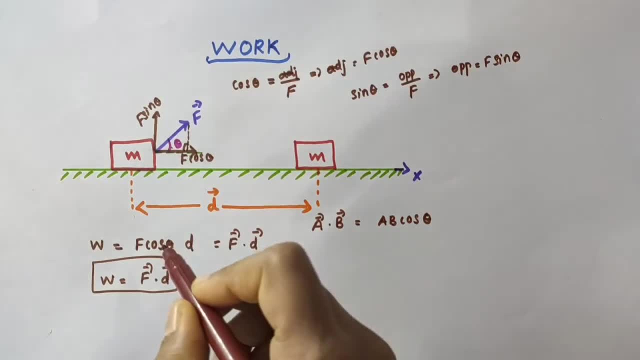 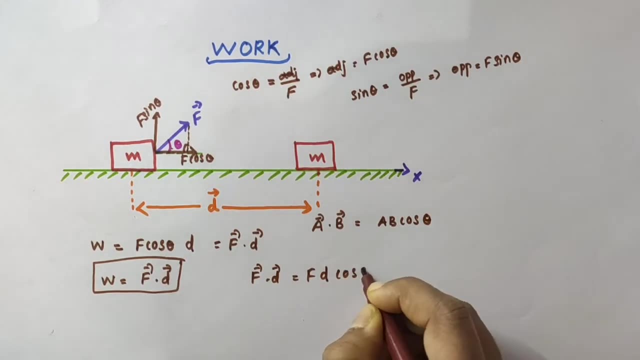 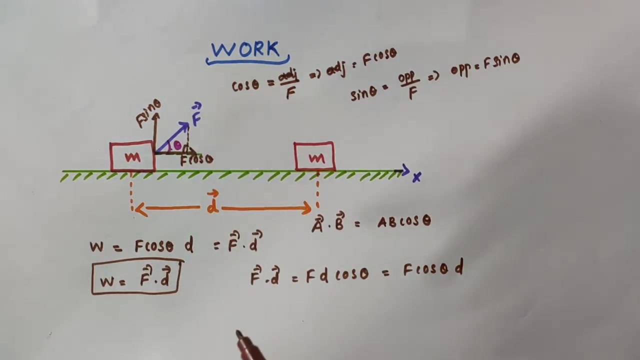 b is equal to a b cos theta. so vector f dot vector d is equal to what? f d cos theta? okay, vector f dot vector d is equal to f d cos theta. or you can write it as f cos theta into d, no problem. or you can write it as f into d cos theta, like that, no problem with that. okay, so you see, it is a scalar. 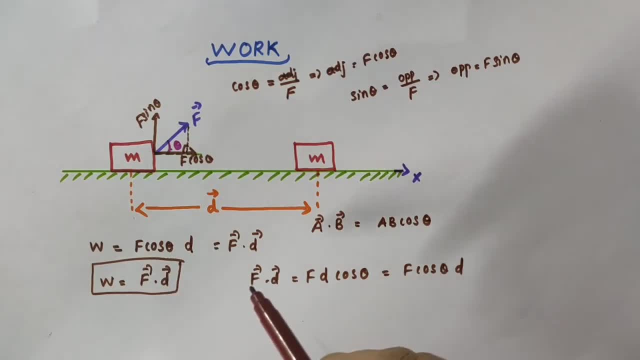 product now. so this f cos theta into d, that can be written as what vector f, dot vector d. so no problem with that. so we can write the work done as the dot product of the force and the displacement. okay, see, force is a vector quantity, displacement is a vector quantity. but when we take the dot. 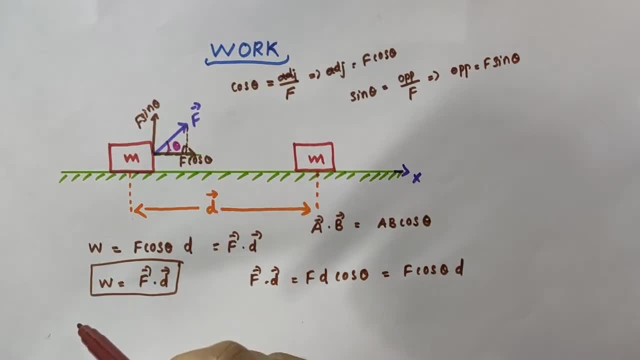 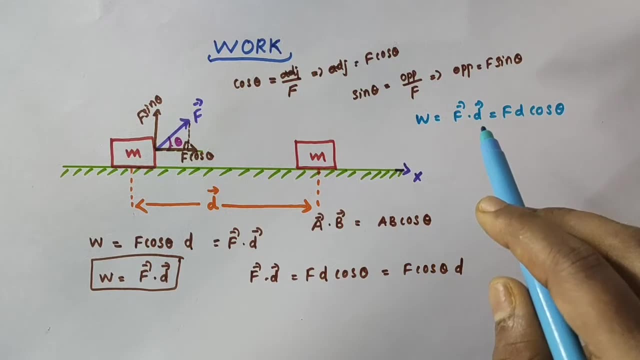 product of these two we are getting a scalar quantity, which is the work done here. so we got: w is equal to work done, is equal to vector f, dot vector d, which is equal to magnitude, force, into magnitude of the displacement, into cos of angle, between vector f and vector d. okay, 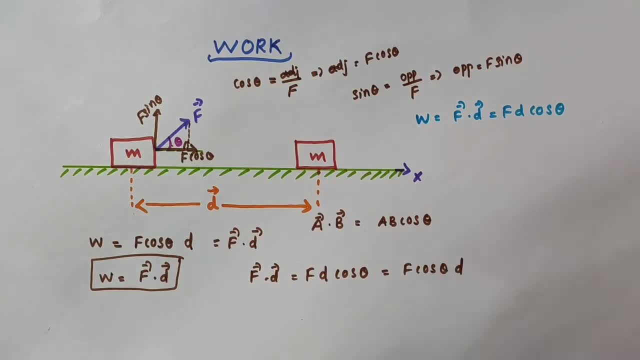 f, d cos theta. now you see, if there is no displacement- no, displacement means magnitude of the displacement, d equal to zero- then there is no work done. no, even if the force is large, okay. if there is no displacement, that is d equal to zero, then there is no work done, even if the 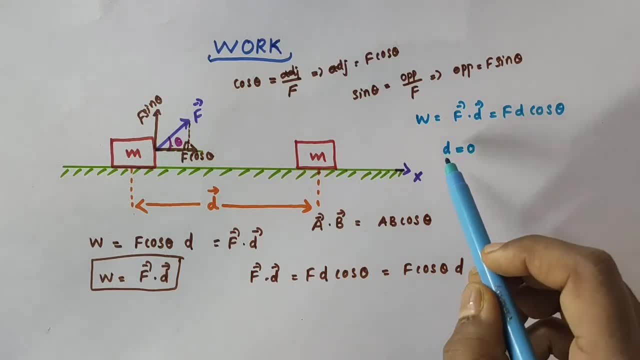 force is large. that is see, when there is no displacement, we can take d equal to zero. so d equal to zero, zero into any value, okay, zero into any value will give you zero, okay. so there can be a force which is very large, but if the displacement is zero, then the product becomes zero. that is, work done is equal. 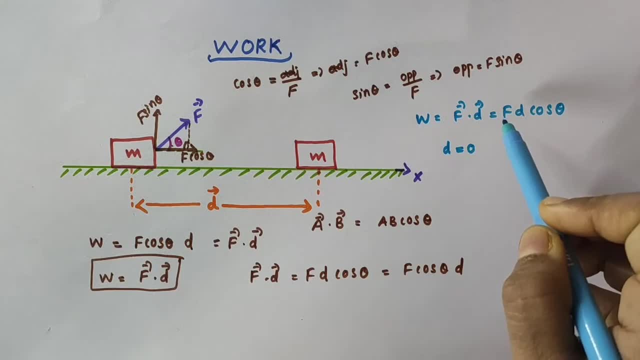 to zero. okay, so whatever be the magnitude of the force, if there is no displacement, the work done will be zero, okay, that is, for example, when we push hard against a rigid brick wall. okay, you just imagine this as a rigid brick wall and we are pushing against very hard on this rigid brick wall. the force we exert on the wall does no work. why, why? 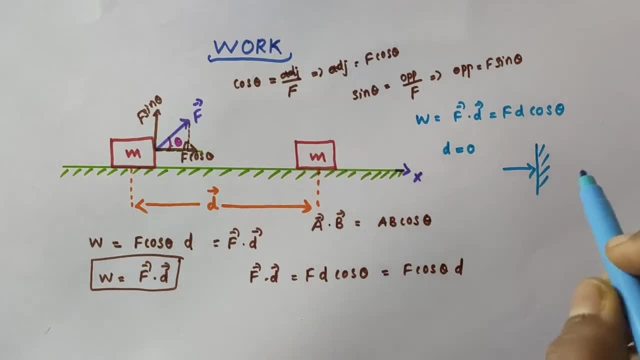 because, though we push the wall with a larger force, the wall will not get displaced. the wall will be there itself. now, okay, so displacement is equal to zero. hence, w work done is equal to zero. okay, but we get tired now because our muscles are alternatively, contracting and relaxing and 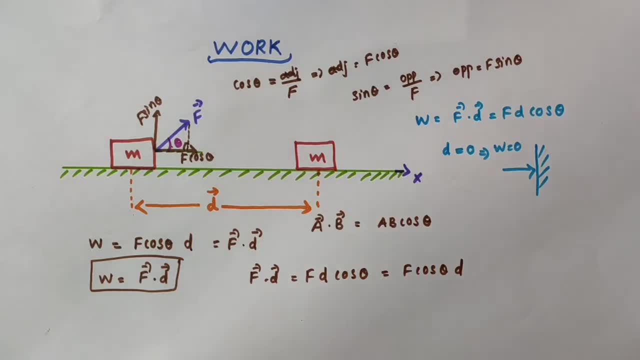 internal energy is being used up and we get tired. so we can say that no work is done if there is no displacement. okay, for example, another one example: a weight lifter. you just imagine he is holding a 150 kilogram mass steadily on his hold. i mean, 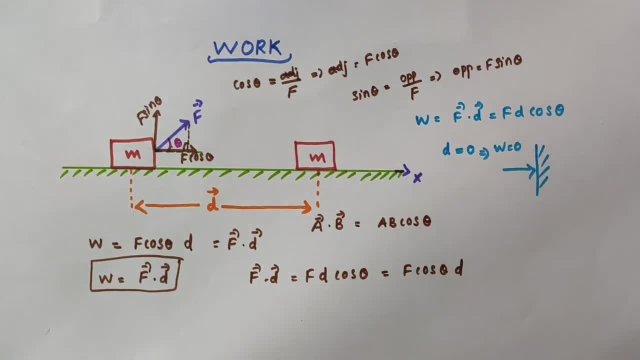 shoulder for 30 seconds or 15 seconds, whatever be the time. he does no work on the law during this time. why why? because, though he applies this- i mean some force on the load- he does not work on the load to hold it. there is no displacement for the lord because he is standing there now that lord is. 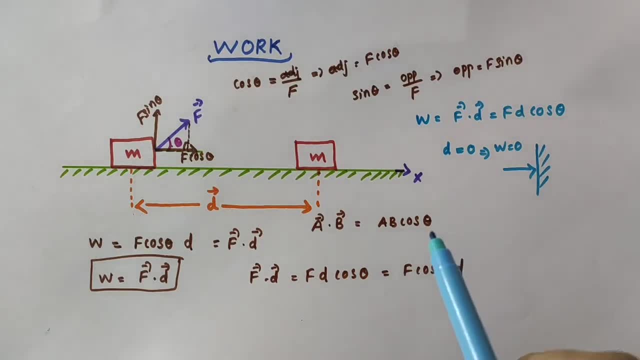 there on his shoulder. there is no displacement for that lord, so displacement is zero in this case. okay. so if displacement is zero, then work done will also be zero. okay, similarly, no work is done if the force is zero. okay, there can be the displacement values, there will be some displacement for the object, but if the force is zero, then no work is done. 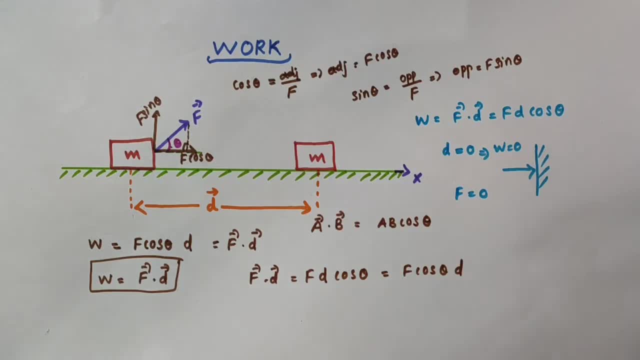 Because 0 into any value will give you 0.. For example, a block moving on a smooth horizontal table- Okay, you just imagine this as a smooth horizontal table, Then there will not be. I mean that block is not acted upon by a horizontal force. 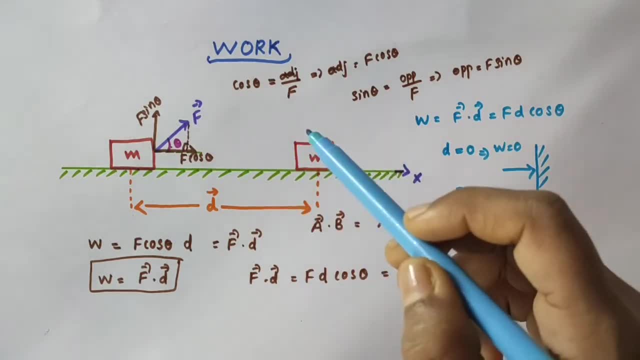 Because it is a smooth horizontal table. no, So there is no friction, since it is a smooth horizontal table. Okay, but the block may undergo a large displacement, Alright. so what will be that? I mean here the force is equal to 0.. 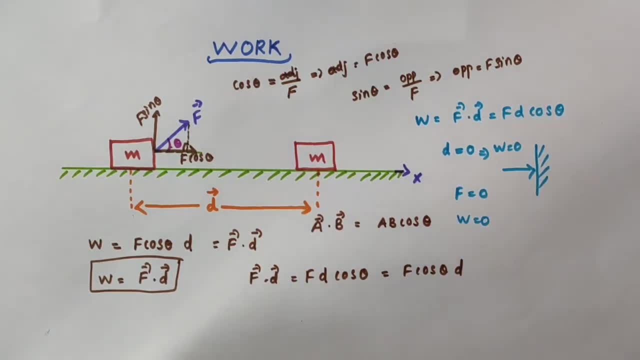 So what about the work done? Work done will be equal to 0.. Okay, when we consider the block moving on a smooth horizontal table, it is not acted upon by a horizontal force. Okay, you just imagine initially, sometimes we may have applied some force on it. 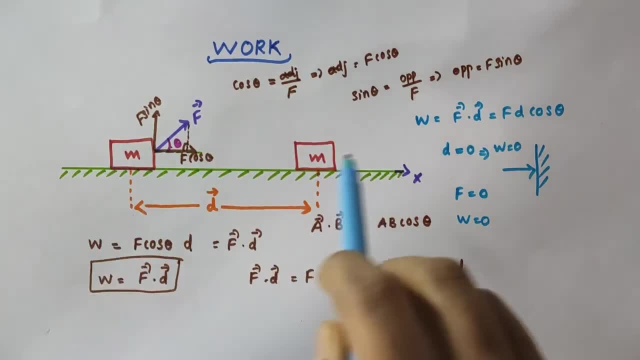 And after sometime, since there is no frictional force, it continues its motion. So we are considering that particular situation. So in that particular situation there is no horizontal force acting on this, This block, because there is no frictional force here. 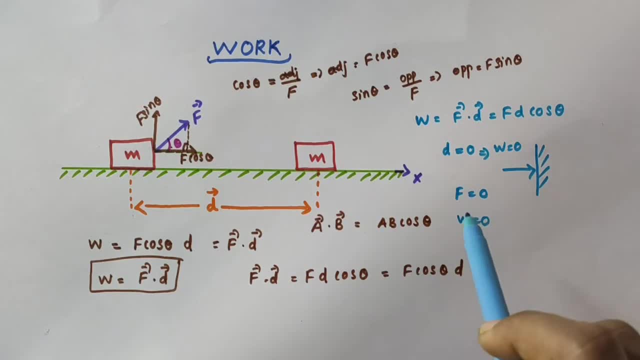 But the block may undergo a large displacement, So in that case force is equal to 0.. So work done will be equal to 0.. Okay, now, no work is done if the force and displacement are mutually perpendicular. Okay, that is, we have work done. is equal to vector F, dot. vector D, which is equal to F, into D, into cos theta. 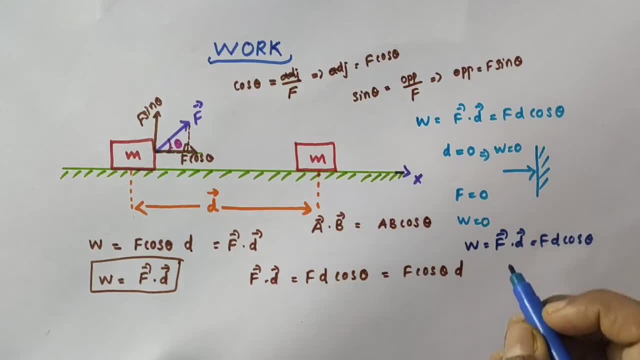 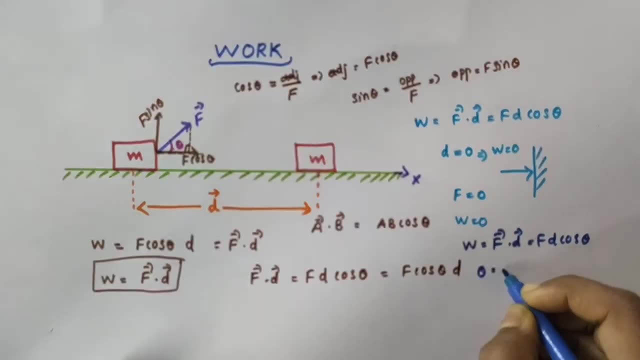 So if this force vector and the displacement vector are mutually perpendicular, mutually perpendicular means the angle between them is equal to 90. That is, theta is equal to 90 degree. So what about the work done, F into, D into, they will have some values, then cos 90.. 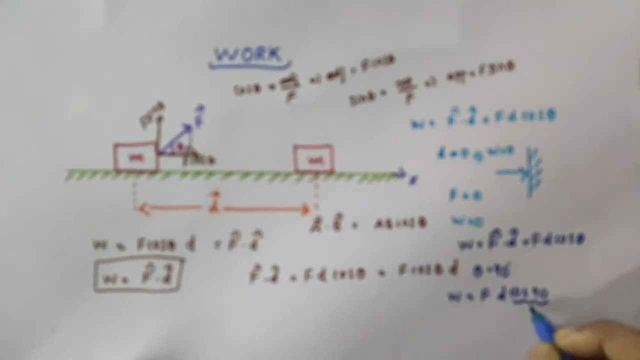 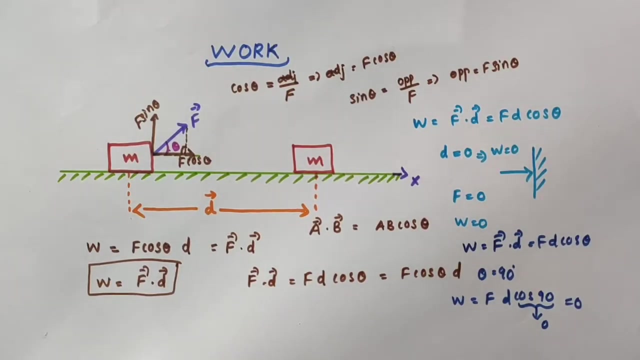 So, whatever be the values of F and D, what is cos 90?? Cos 90 is 0, no 0 into any value will give you 0. So work done is equal to 0. Okay, that is no. work is done if the force and displacement are mutually perpendicular. 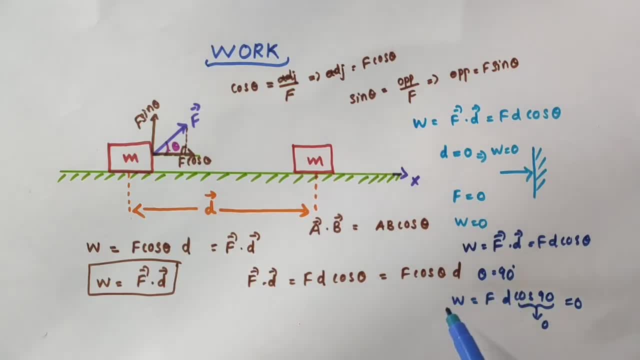 Okay, mutually perpendicular, Okay, mutually perpendicular. Theta is equal to 90. So W is equal to F into D, into cos 90. Whatever be the values of F and D, cos 90 is 0.. 0 into any value will give you 0. 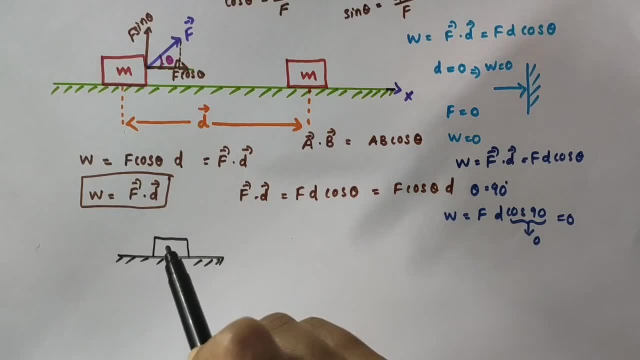 For example, for a block moving on a smooth horizontal table. this block is of mass m, It is moving on a. you just imagine it is moving along this direction on a smooth horizontal table. Okay, there is no horizontal force acting on it. 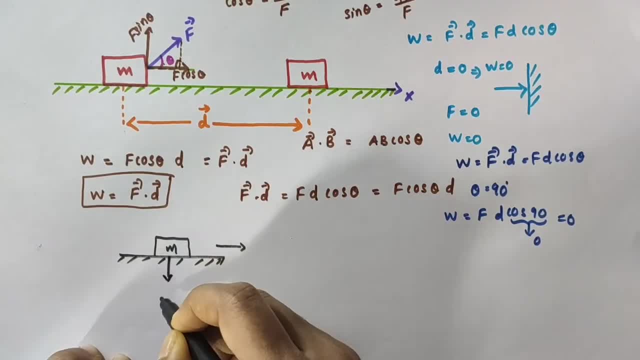 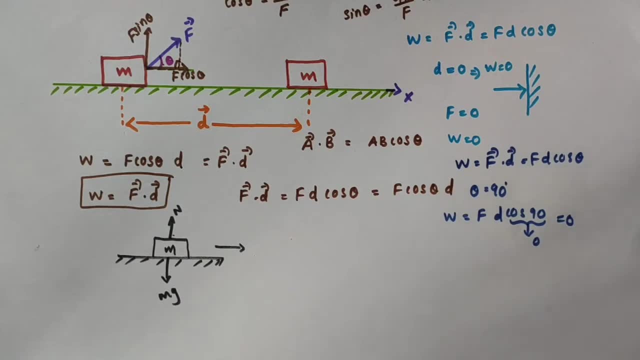 All right, but there are gravitators, Gravitational force which is acting in the vertically downward direction, and there is a normal reaction force which is acting in the vertically upward direction. Alright, but you see, here we can say that, or here, if we are considering the work done by the gravitational force, what will be that work done by the gravitational force? 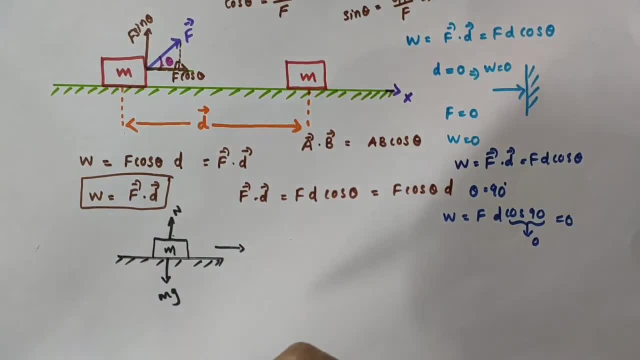 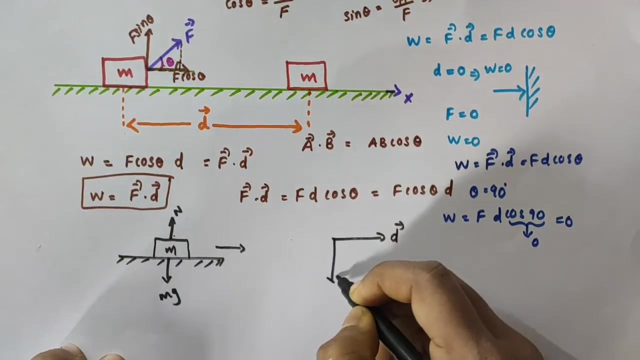 See, gravitational force is acting in the vertically downward direction. So here we can say that the gravitational force Mg does no work. Why See, the displacement is along this direction. okay, displacement is along this direction and the gravitational force it is acting along this direction, that is, in the vertically downward direction. 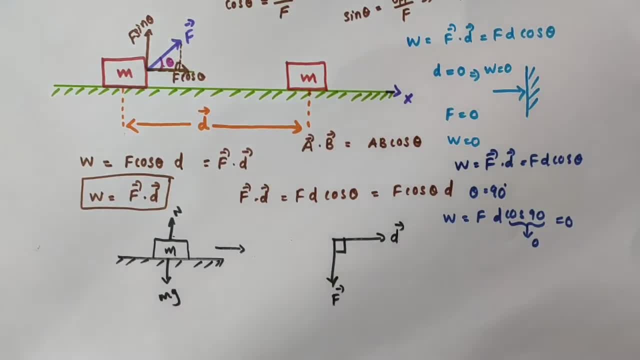 Alright, so what is the angle between this gravitational force and the displacement vector? That is 90.. Okay, so theta equal to 90, cos 90 equal to 0, 0 into any value will give you 0.. Okay, so the gravitational force does no work since it acts at right angles to the displacement. 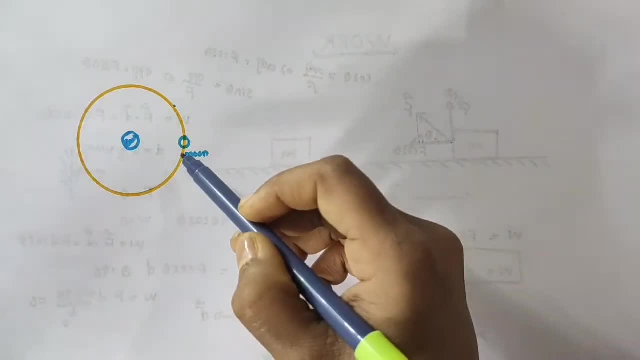 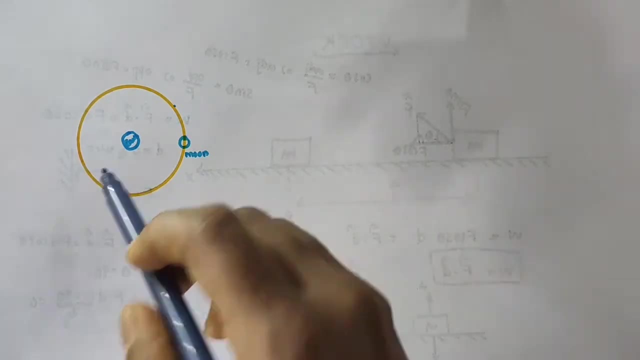 Now, if we assume that the moon's orbit around the earth is perfectly circular, then the earth's gravitational force does no work. You just imagine this as the earth and the moon is orbiting around the earth through a circular orbit. So we are just assuming that the moon's orbit around the earth is a circular, perfectly circular orbit. 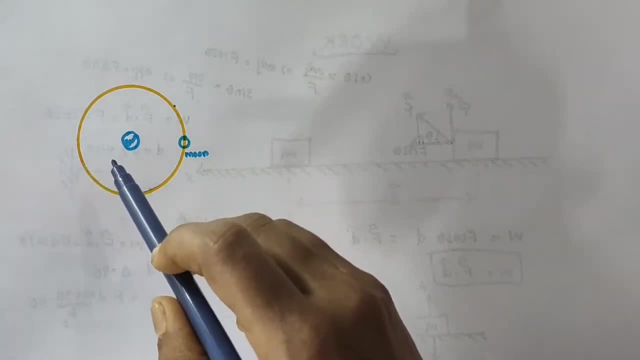 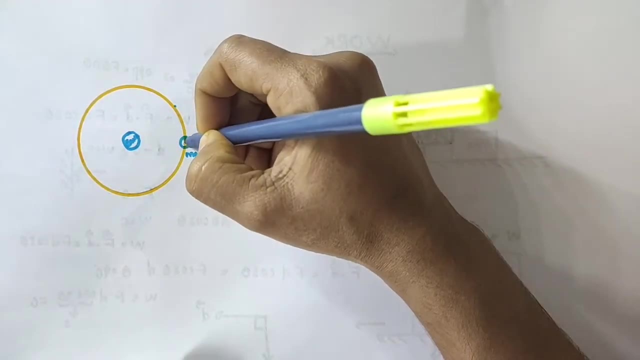 So in that situation, the gravitational force, the earth's gravitational force, does no work, Because you see, the moon's, this instantaneous displacement, that is, when the moon is somewhere here, its displacement at that particular time will be along the tangent. 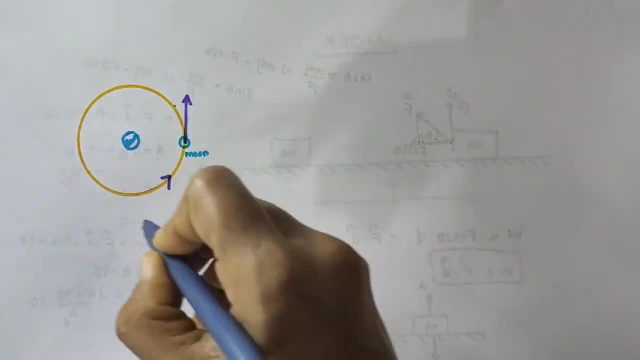 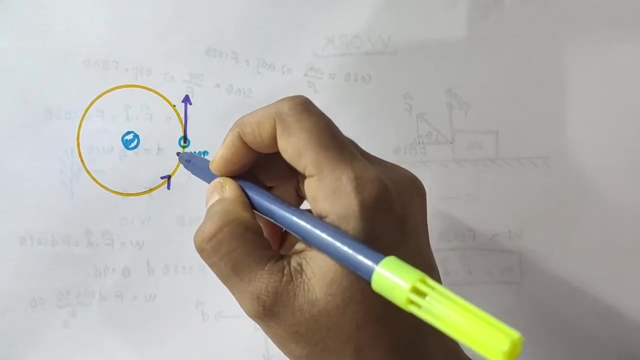 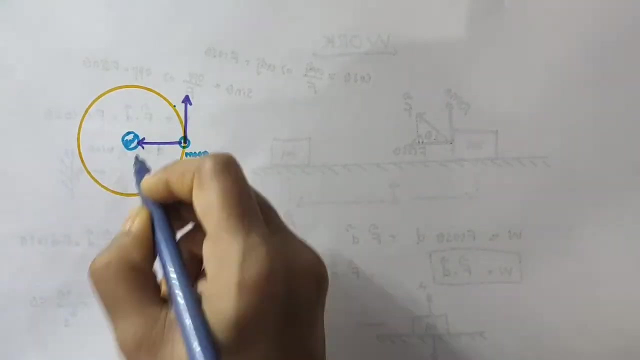 You just imagine the moon is. I mean, the moon is orbiting in this particular direction. So this will be the instantaneous displacement vector of this moon at this particular point. Okay, and you see the earth's gravitational force that is acting towards the earth's center, no, or center of the circular part, no, 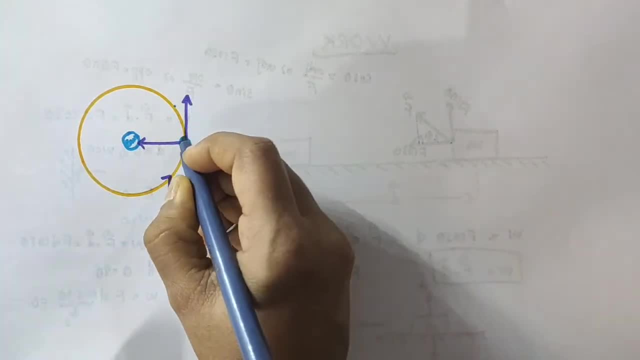 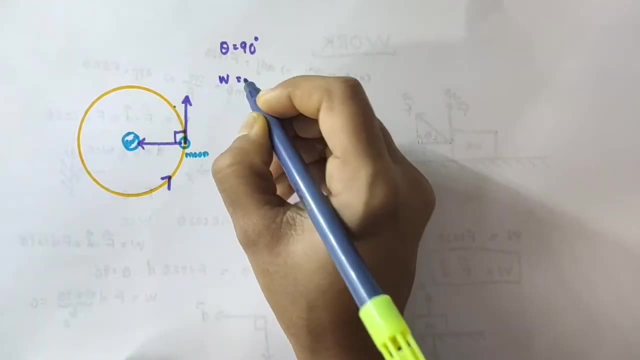 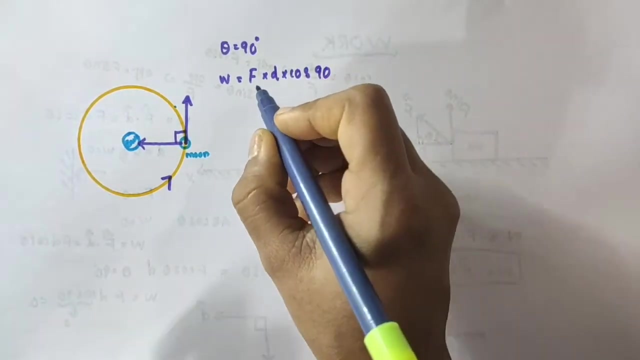 So force is acting along this direction and displacement is along this direction. so what is the angle between them? theta equal to 90. okay, so what about the work done by the gravitational force? gravitational force into displacement, into cos. self angle between them that is 90. so whatever be the magnitudes of f and d, cos 90 is 0. so 0 into any value will give you. 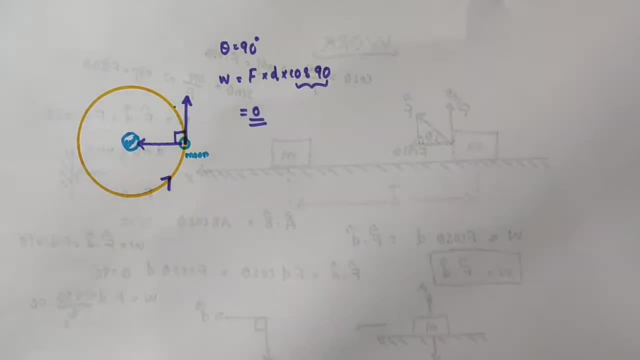 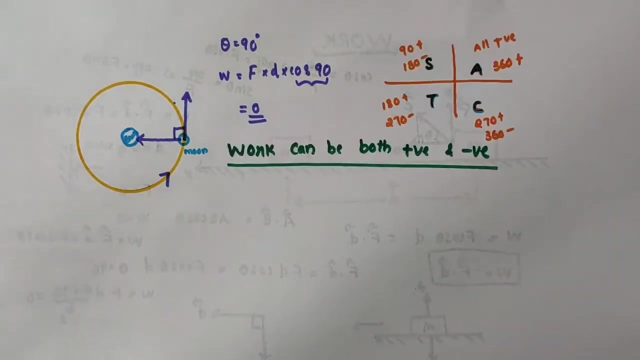 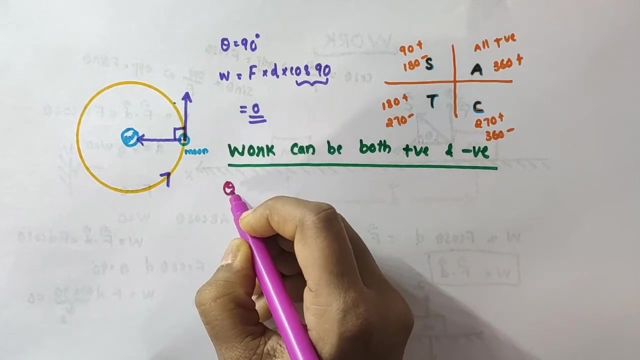 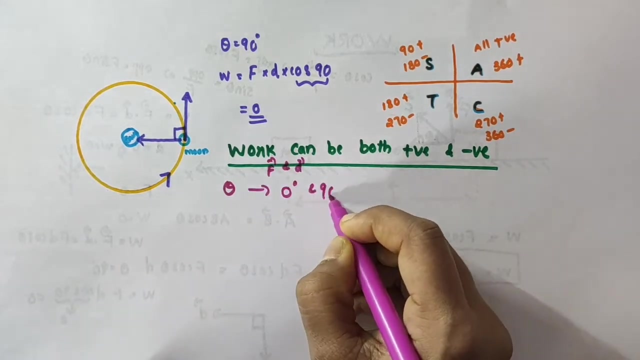 0. okay, so we can say that the gravitational force, the earth's gravitational force, does no work. all right, now, work can be both positive and negative, that is, if theta, which is the angle between vector f and vector d, is between 0 degree and 90 degree. okay, if theta is between 0 degree and 90 degree, then 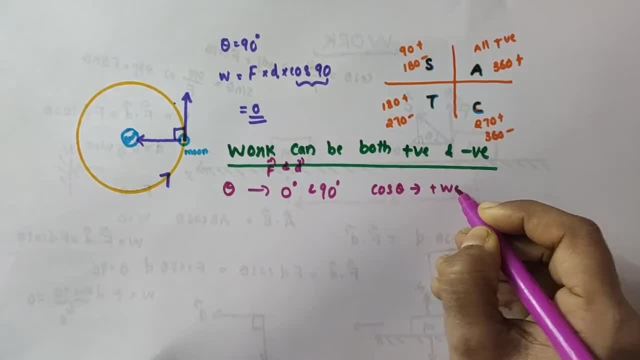 cos theta is positive, hence the work that is, then work done also will be positive. okay, if theta work done can be positive as well as it can be negative, then it can be positive as well as it can be negative if theta is between. that is, theta is the angle between vector f and vector d. 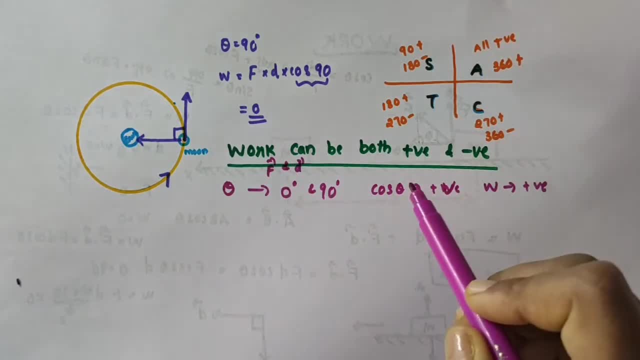 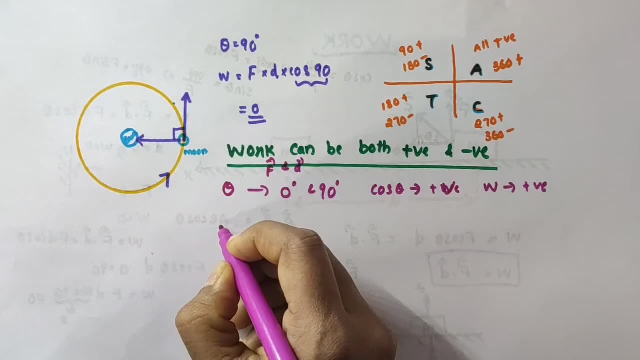 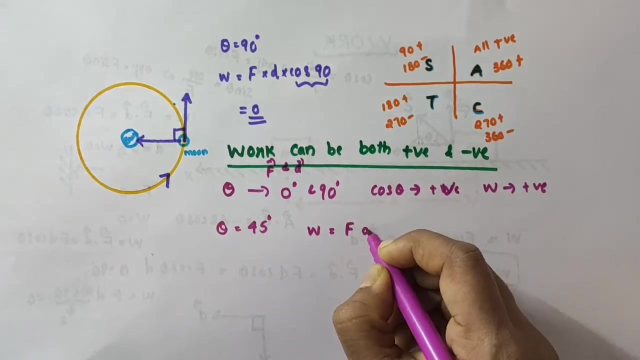 if theta is between 0 degree and 90 degree, then cos theta will be positive. so work done will be positive. okay, for example, let us take theta is equal to 45 degree. okay, so what about the work done? we can write the work done as magnitude of force, into, magnitude of displacement, into. 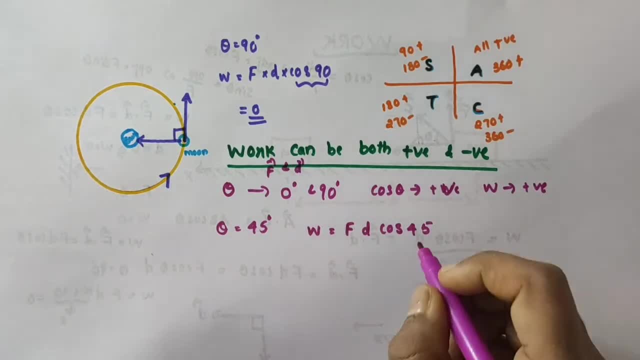 cos of angle between them, that is cos 45. what is the value of cos 45? that is 1 by root 2. no, okay, that is F into d, into one by root 2. so magnitude of F, magnitude of d and 1 by root 2, all. 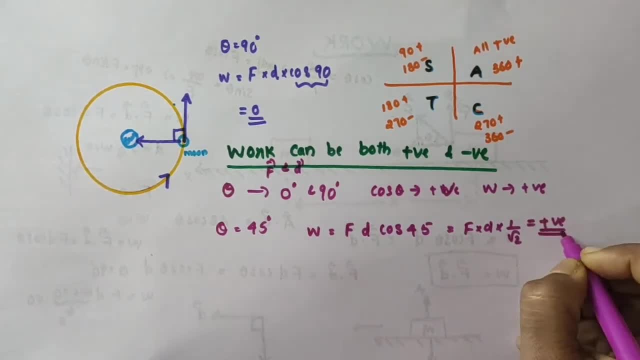 are positives now. so this will be a positive quantity. that is work done as positive when theta is between 0 degree and 90 degree, because 45- here we have taken theta as 45 degree, which is between 0 degree and 90 degree now, so work done will be positive. okay now if theta is between: 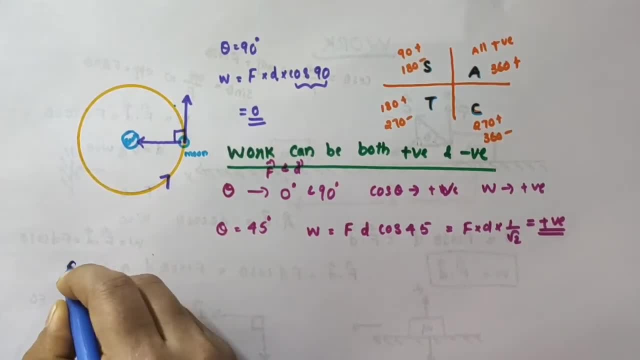 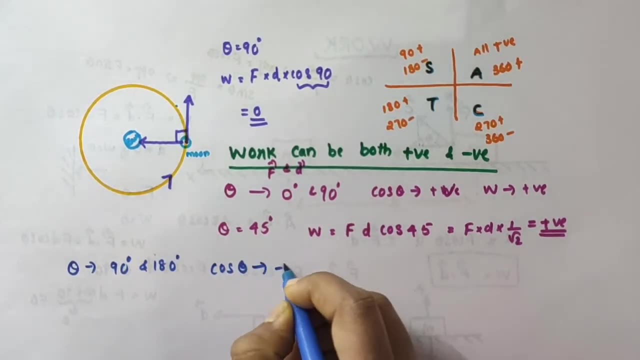 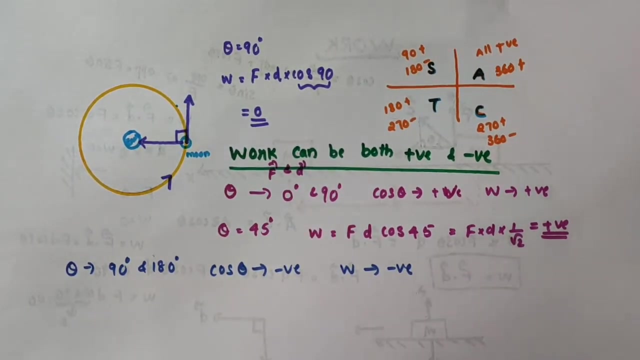 90 degree and 180 degree. okay, if theta is between 90 degree and 180 degree, then cos theta will be negative. hence, work done: ok, work done also will be negative, alright. for example, let theta is equal to 135 degree. ok, so what about the work done? w is equal to magnitude of force, into magnitude of displacement, into cos of 135. 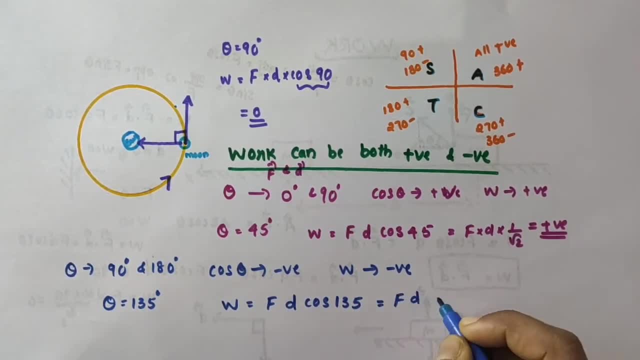 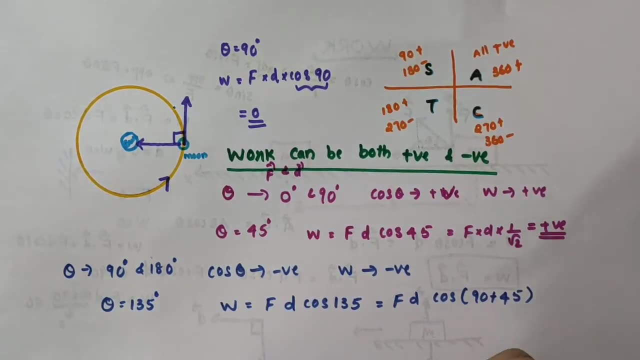 how can we find out cos of 135 f into d, into cos of 135 can be written as cos of 90 plus 45. no, ok, 90 plus 45 is what 135? alright, now you have studied about this. no a, a, s, t, c here, all i mean. 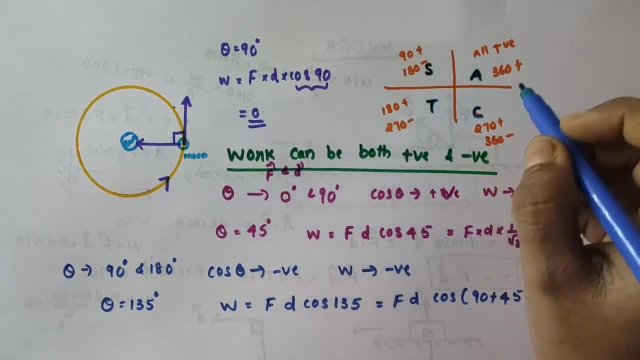 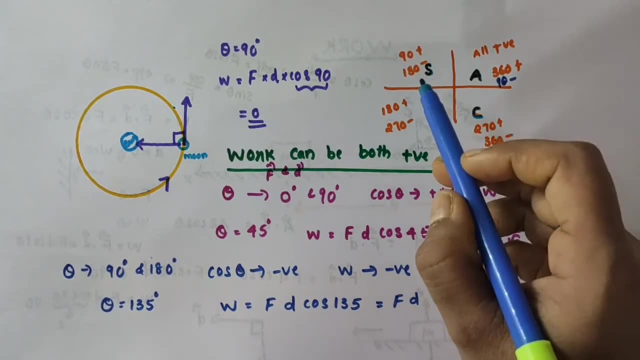 in this quadrant. all i mean this quadrant is actually. i mean, this quadrant is actually 90 minus values and 360 plus values, and all are positive here. this is sine is positive here, right, this is for 90. positive here. right, this is for 90. positive here. right, this is for 90. 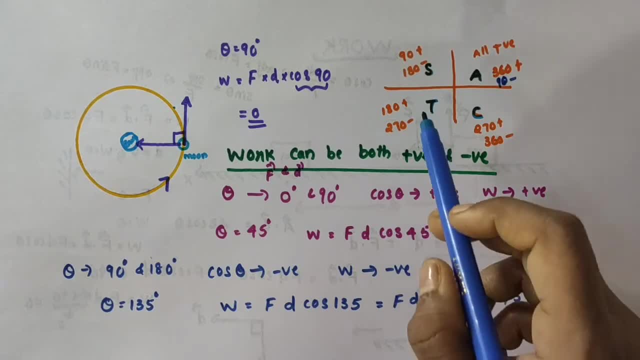 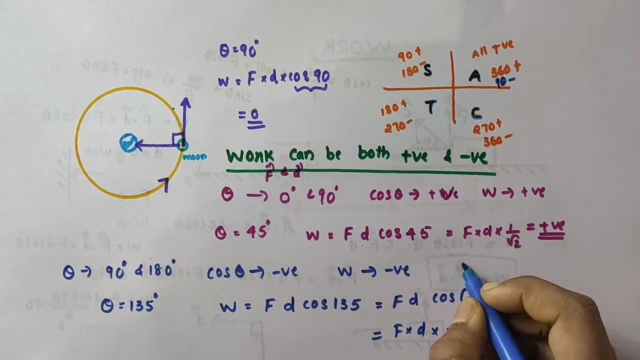 plus and 180 minus, like this. so here we have cos of 90 plus 45. 90 plus will come in this quadrant and here cos is negative, actually ok, so this actually becomes f into d, into minus, cos theta, that is minus. i mean cos of 90 plus theta is actually ok, you have studied this cos of 90 plus. 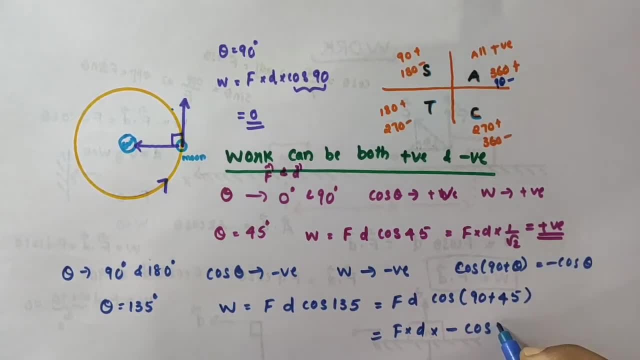 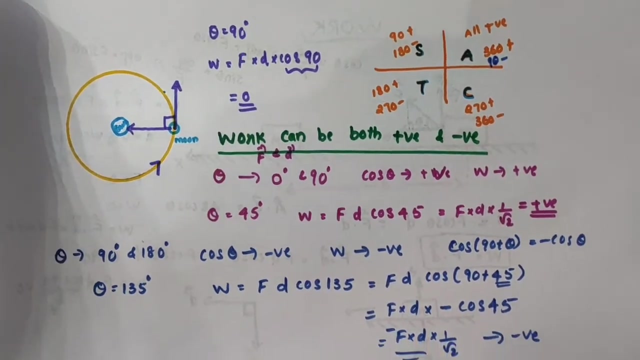 theta. this is actually minus cos theta, so this becomes minus cos theta is 45 degree. alright, so f into d into cos 45. negative is 1 by root 2 but 1 negative sign here. so you see work done is negative. ok, so this work done can be positive as well as it can be negative. 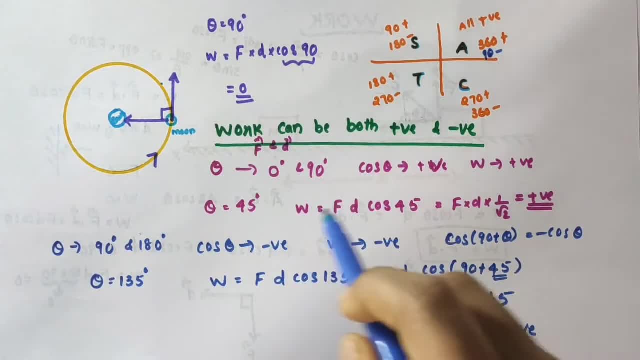 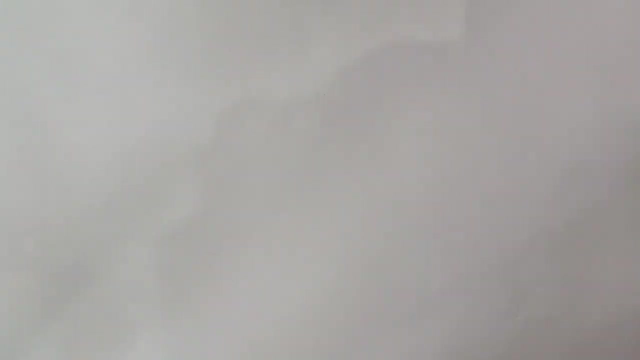 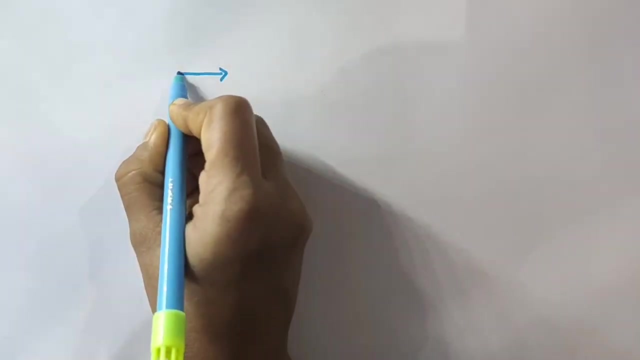 if theta is between 0 degree and 90 degree, then work done is positive. if the theta is between 90 degree and 180 degree, then work done is negative. now what about the work done by the friction? friction opposes the displacement of the object. no, That is. if the block moves along the positive x direction, then the friction will be along. 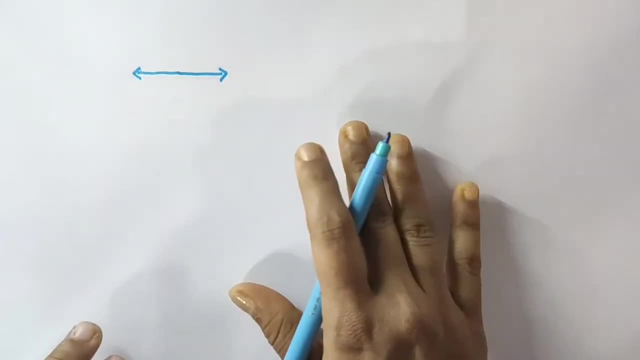 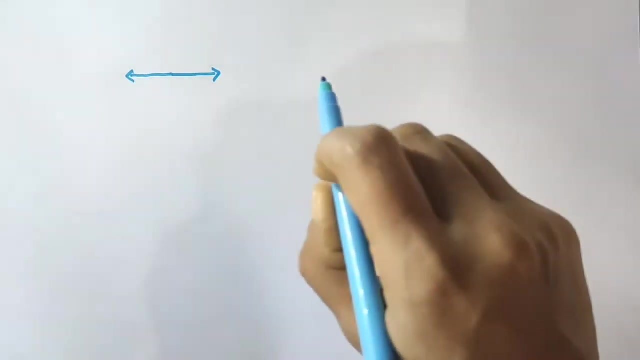 the negative x direction because friction opposes displacement right, or friction opposes the motion of the object. So if the block moves along the positive x direction, that is, if the displacement of the block is along the positive x direction, friction will be against that. opposite to that that. 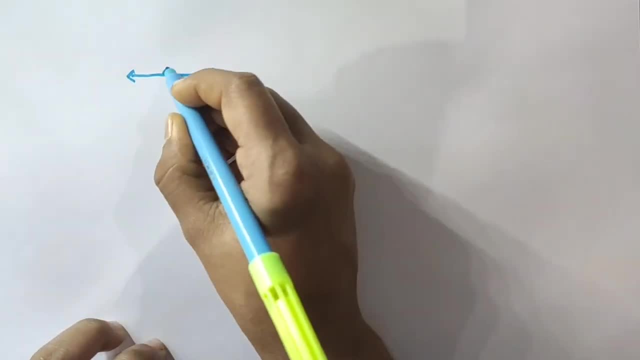 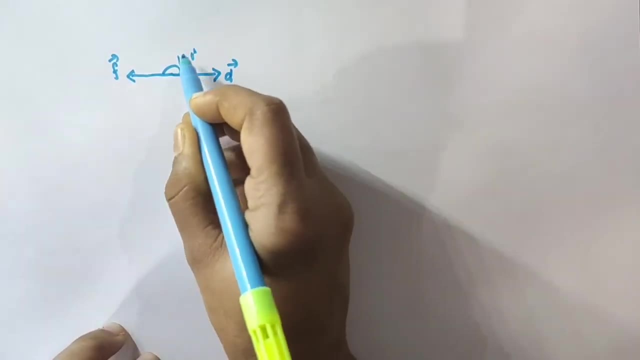 is friction will be along the negative x direction. So what is the angle between? the? displacement is along this direction, frictional forces along this direction. So what is the angle between them? 180 degree, Okay. so what about work done here? work done is equal to magnitude, of force into magnitude. 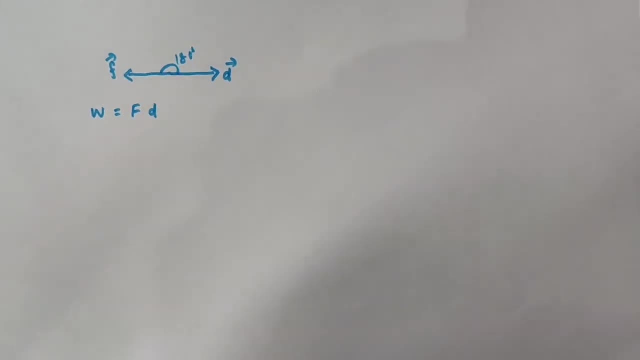 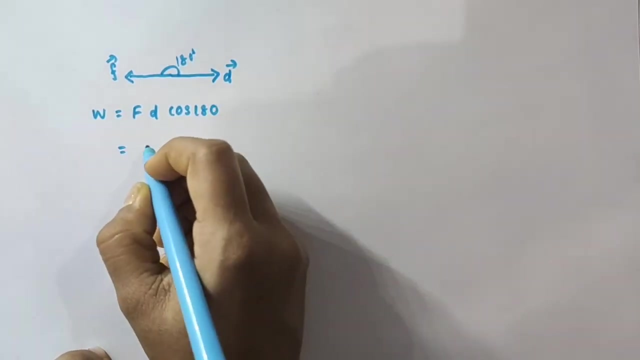 of displacement into course of angle between them. So what is that? angle between vector f and vector d? 180 degree. So course of 180. okay, course, 180 is minus 1 now. So work done will be minus f into d, that is, work done will be negative. 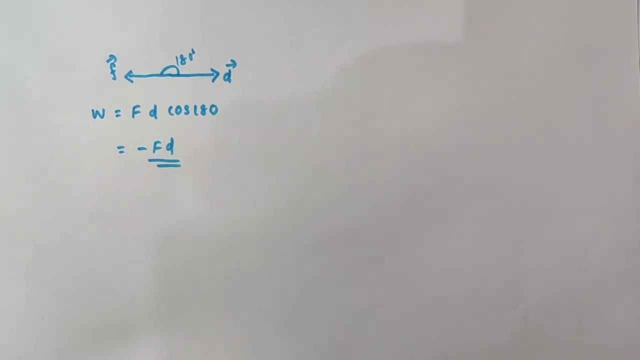 All right, now what about the dimension of work? How can we find out The dimension of work? we have this formula and also we can easily find out the dimension. Okay, so dimension of work will be what dimension of force? force is mass into acceleration. 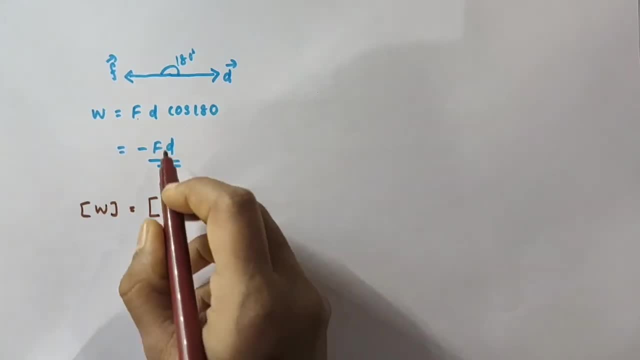 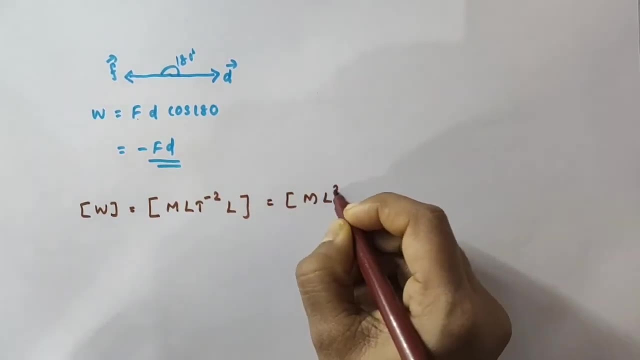 So m dimension of acceleration is l t raised to minus 2, then displacement is l. We don't want to take care of this course actually, So this becomes m, l l l square t raised to minus 2.. So m l square t raised to minus 2 is the dimension of work. 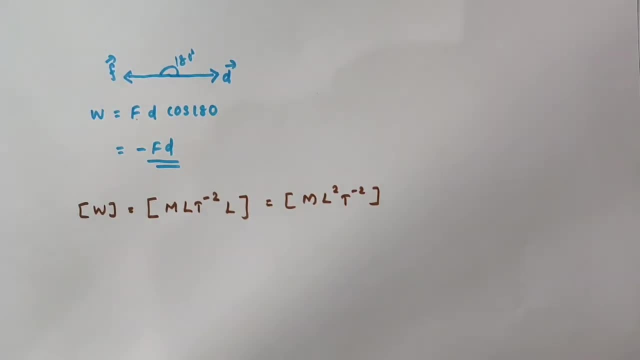 Now, what about the dimension of energy? So to get the dimension of energy you can take any equation of energy, but I am just taking the famous equation: e is equal to m c square, So dimension of energy is equal to dimension of mass, that is m. then dimension of c is the speed of light? no. or velocity of light in vacuum: no. 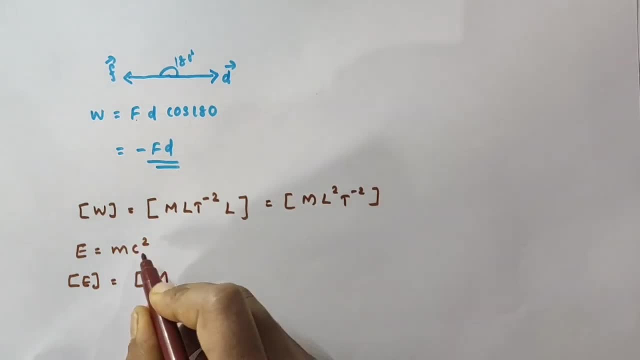 So it is the dimension of velocity. dimension of velocity, square is here, okay. dimension of velocity is l? t raised to minus 1, but square is here, so all square, So l square, then t raised to minus 1. all square means t raised to minus 2..